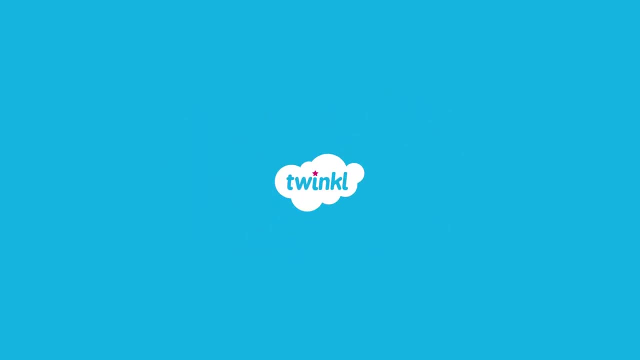 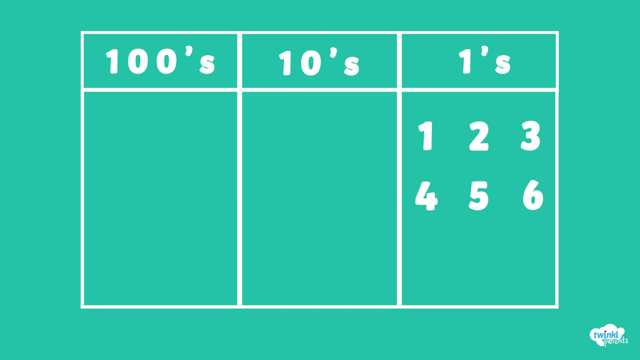 This video will help to explain how place value works. Place value is the value of each individual digit within a number. Let's have a practical look at how this works. So we start out with the 1s. Let's count 1,, 2,, 3,, 4,, 5,, 6,, 7,, 8,, 9, but what about 10?? Where? 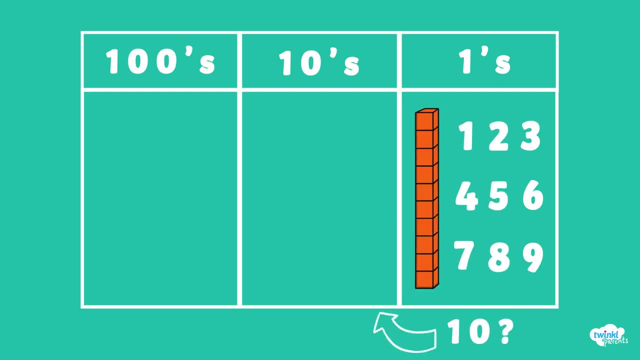 does that belong? You can't have more than 9 1s, So we group them together to make 10 and move them into the 10s column. Continue to add the 1s 20.. 30., 40.. 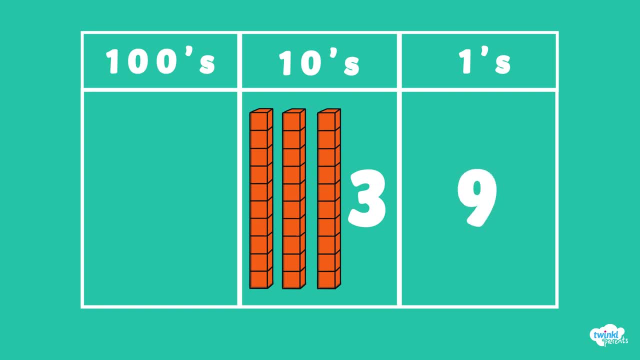 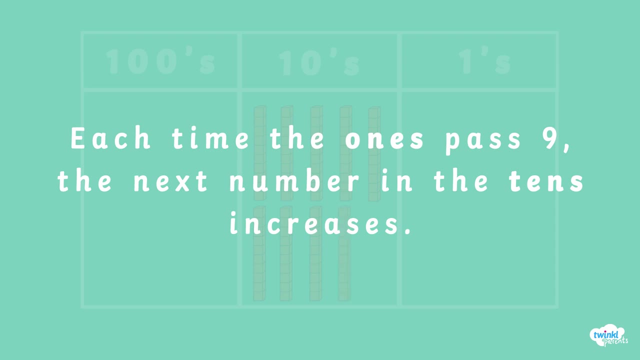 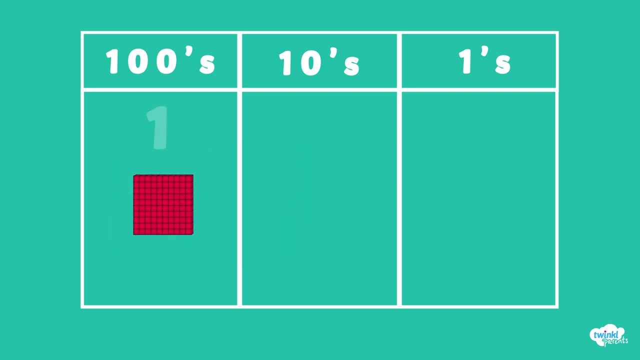 Each time with 1s past 9,, the next number in the 10s increases When you hit 99. we are then introduced into the 100s column. We group the digits together, 0,, 16 and Tends together to make a hundred and move across into the hundredth column. 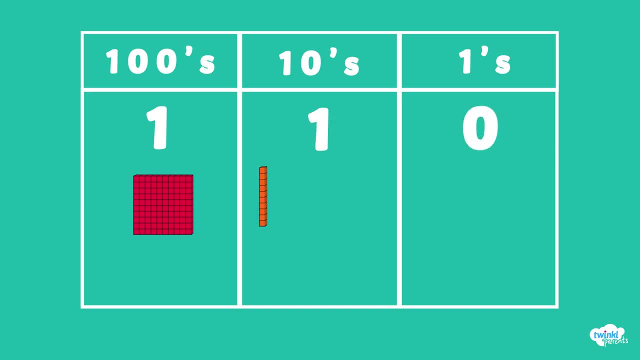 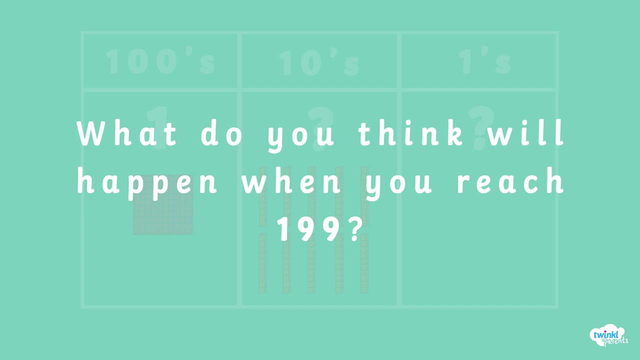 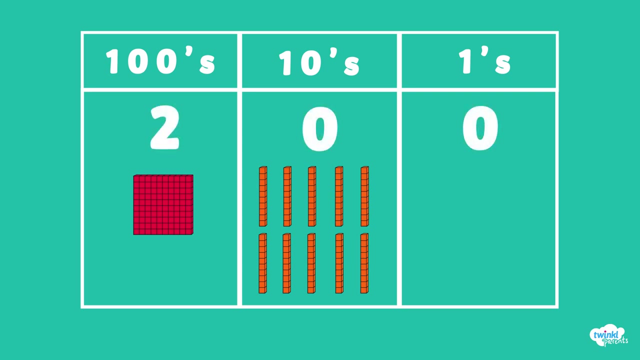 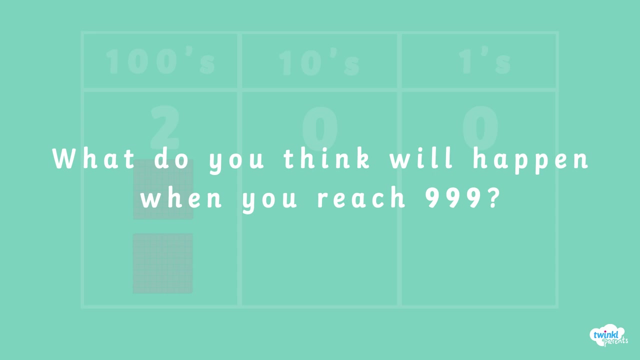 Now it's time to add the worms. What do you think will happen when we reach 199?? We group the tens together to make another hundred and move this one across to the hundredth column. This will now make 200.. What do you think will happen when we reach 999?? Subtitles by the Amaraorg community.